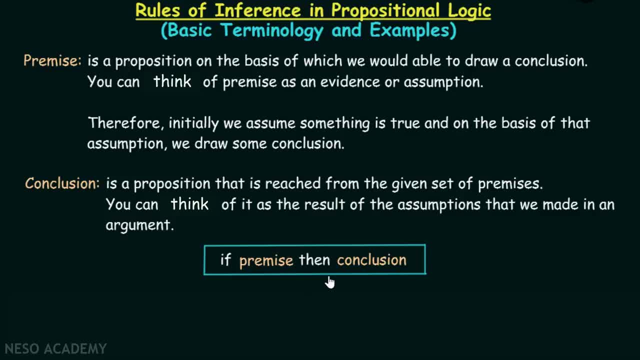 Now we already know what is compound preposition: if P, then Q. Here P is the premise and Q is the conclusion. We know that if premise is true, then the conclusion also must be true. Right, Let's consider the third term, that is, argument. 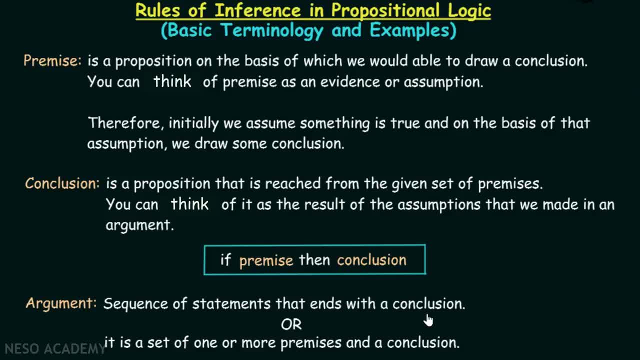 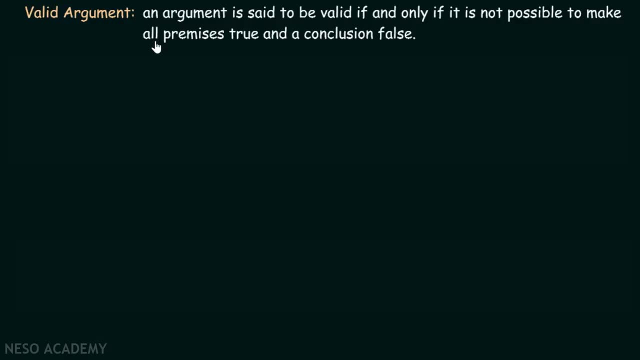 Argument is a sequence of statements that ends with a conclusion, Or It is a set of one or more premises and a conclusion- Simple. Now let's talk about what is a valid argument. An argument is said to be valid if, and only if, it is not possible to make all premises true and a conclusion false. 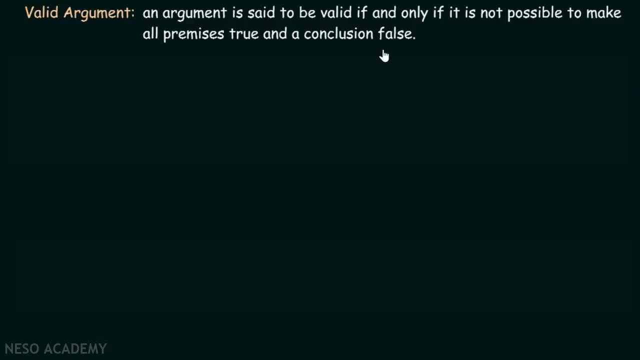 That is. it is not the case that if P is true then Q is false. If P is true, then Q has to be true Right Now. let's consider one example of an argument. If I love cat, then I love dog. 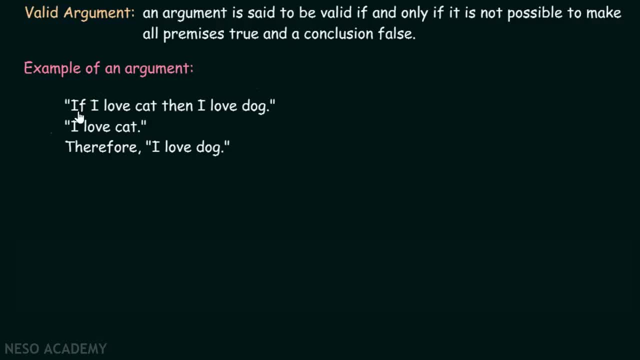 I love cat, Therefore I love dog. Now, this is the first premise. Let's say it is P1.. This is the second premise. Let's say it is P2.. And this is our conclusion, That is indicated by: therefore. 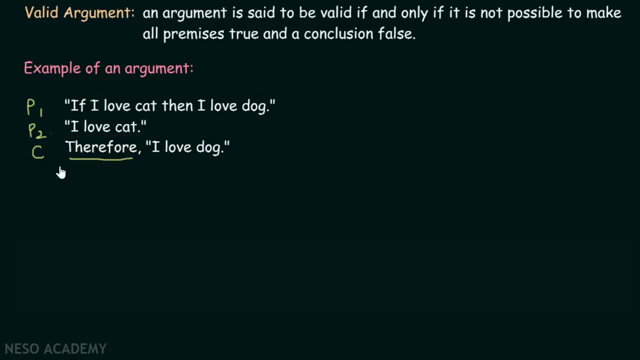 Hence, I love dog is a conclusion. Right Now, let's say: I love cat is represented by P and I love dog is represented by Q. Now, this statement is of the form. P implies Q. Right, This is simply P, and here this is Q. 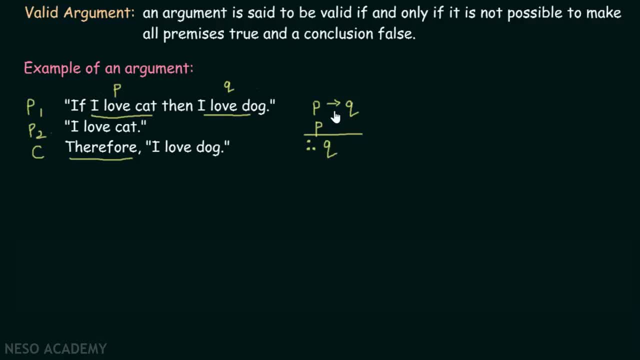 So we can write this argument as P implies Q, then P, therefore Q. We can also write this argument as P implies Q and P implies Q. P implies Q. These are the two premises and this is the conclusion. Premises implies conclusion. Okay Now. 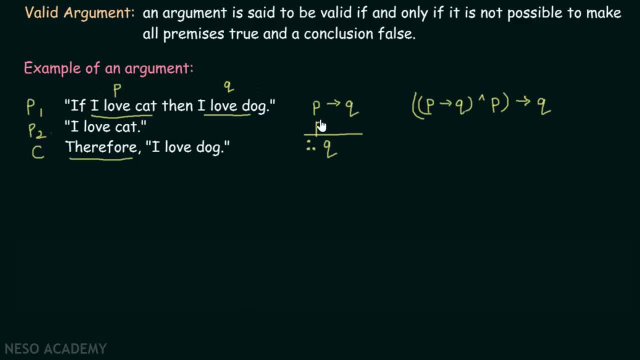 this conclusion can be true or this can be false. It depends on the premises, Right? We initially assume that all these premises are true And in order to prove that this argument is a valid argument, we need to make this conclusion true, Because all premises are true. 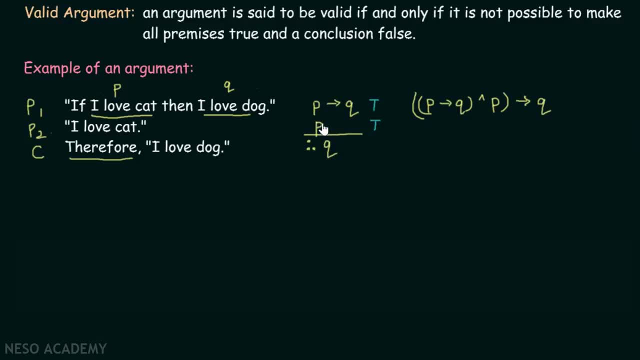 therefore conclusion must also be true. As P is true, therefore here also P is true. And if P is true, then Q must also be true In order to make this compound preposition true. We cannot make this Q false If we make this false. 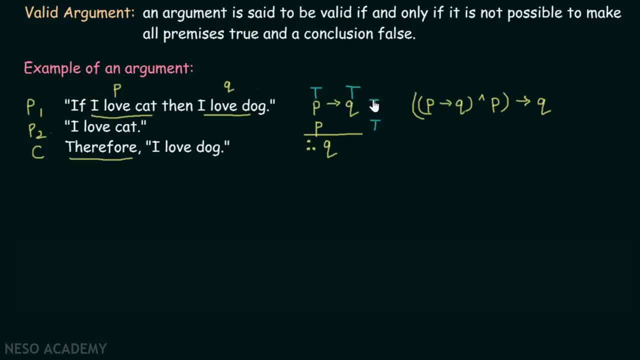 then this whole compound preposition becomes false, Which is against our assumption Right. Hence Q must be true. And if Q is true, because our conclusion is Q only, hence this conclusion is also true, As there is no way we would be able to make. 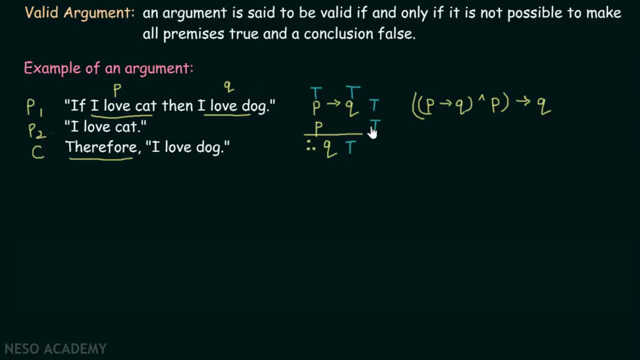 conclusion false by taking premises true And hence we can say that this argument is a valid argument, Right? This is just another way of representing this argument. P implies Q and P. Why I am writing and over here? Because these two premises must be true. 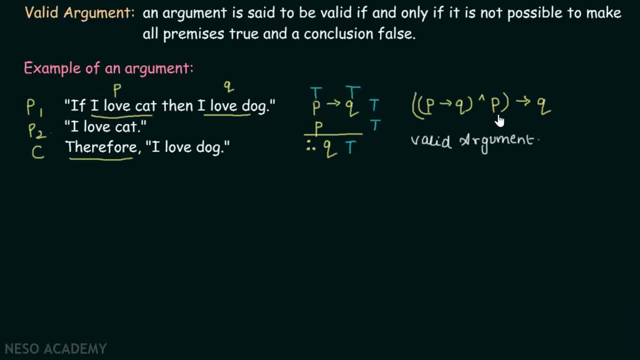 Right. It is not the case that one premise is true and the other one is false, So these two premises must be true and conclusion must also be true, So we can conclude that this whole argument is a valid argument. Let's consider one more example. 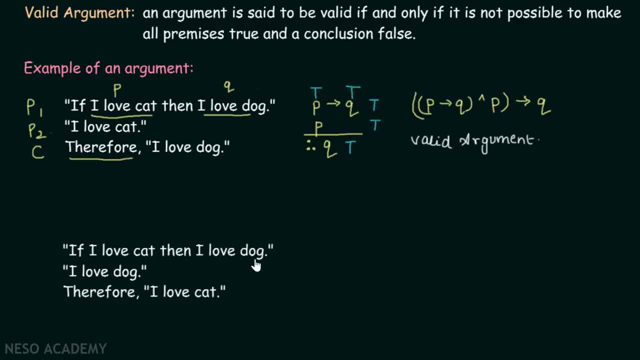 Here I am saying: if I love cat, then I love dog. Second premise is: I love dog and the conclusion is: I love cat. As this statement is of the form implies Q. I love dog, is Q therefore P because I love cat is P. Can we say if P implies Q is satisfied. 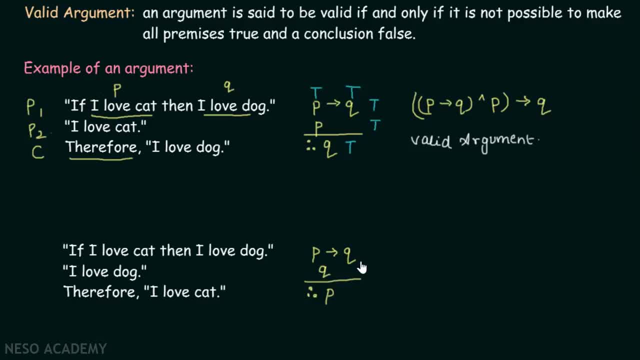 and Q is satisfied, then P is also satisfied. Let's see, Initially we assume that P implies Q is true and Q is also true, And we need to prove that P must also be true. Then only we can say: this argument is a valid argument. 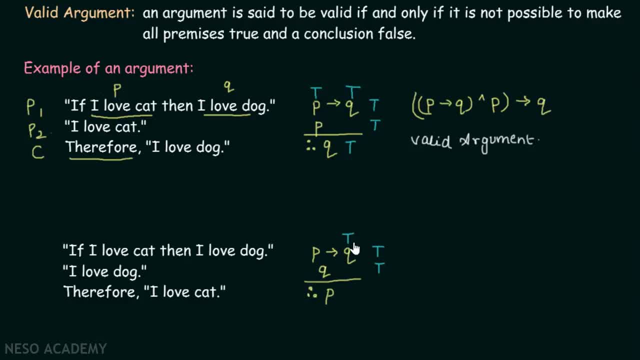 Now, as Q is true, then here also Q is true. and if Q is true, then P can be true or P can be false. If P is false, then false implies true is true. And if P is true, then true implies true is also true.